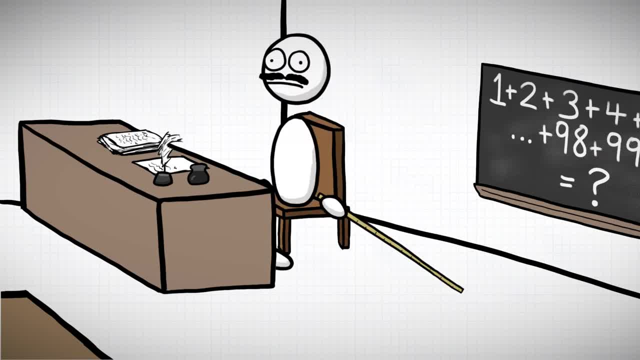 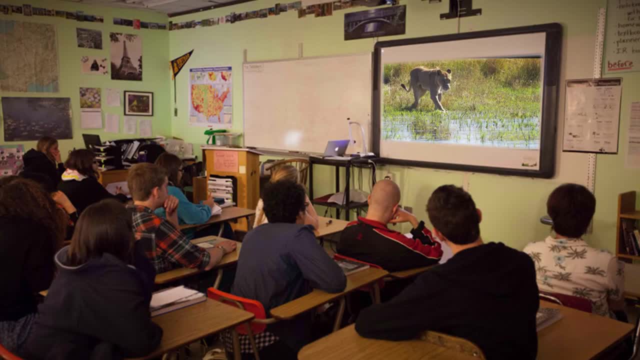 Not as a real lesson, mind you. He just wanted to keep them busy for a bit so he could work on his novel. I guess it's kind of like today when your teacher puts on Planet Earth in science class Or Air Bud in phys ed, So everyone quietly gets to work. 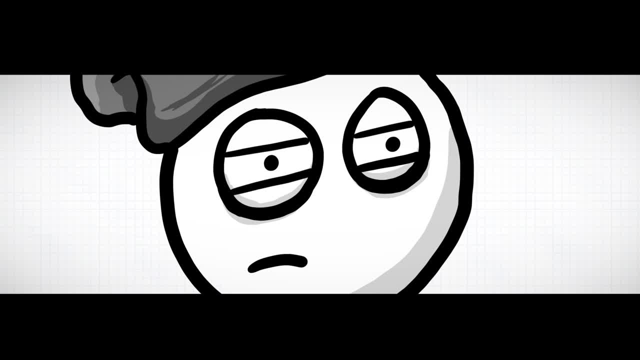 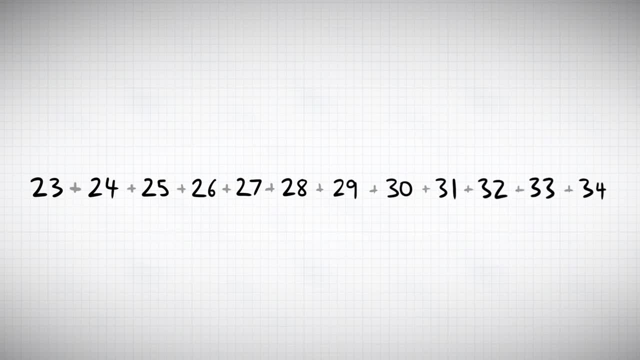 But Carl Gauss was like no bitch And he came up with an easier way to do it. The key to figuring it out was noticing that if you have a sequence of numbers like this and you add the first and the last numbers, they add up to the same thing as adding up the second and second-to-last numbers. 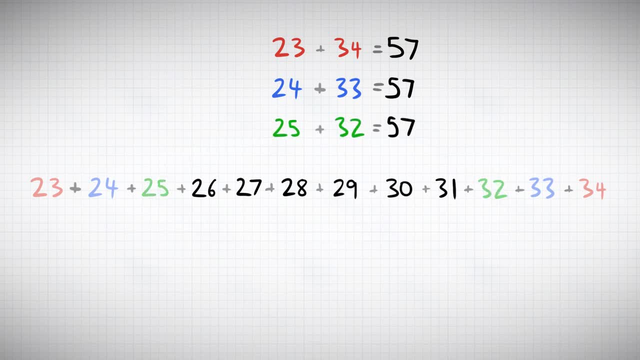 And the same thing goes for adding up the third and third-to-last. This number is one bigger than the one we just did and this number is one smaller than the one we just did. So if we add them together, it's going to be one bigger and one smaller than the sum we. 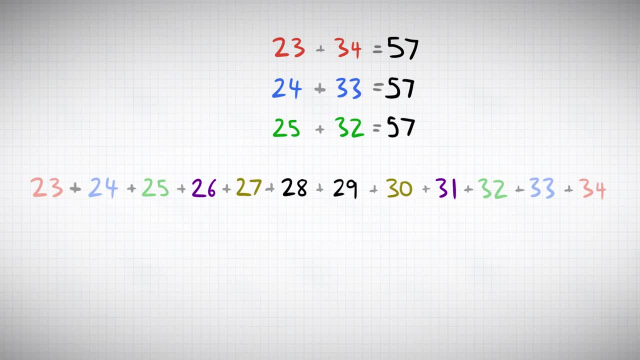 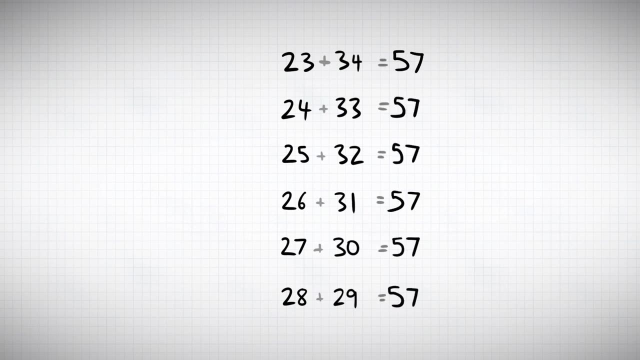 just did So we're going to get the same number And that works all the way to the middle. We can. we can basically just fold the number line in half and all the pairs are going to add up to the same number. Playing with the numbers like this is the secret to adding them up really fast. 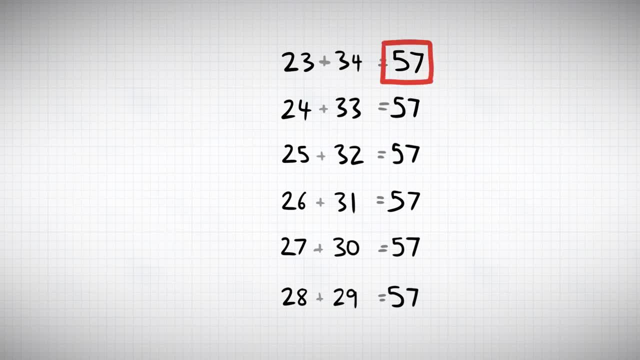 because it lets us multiply this number, the value of the pairs, by the number of pairs, And it's exactly the same as if we had added them up one by one. We're just sort of adding them up in a different order. So for our equation we want to take the first number. 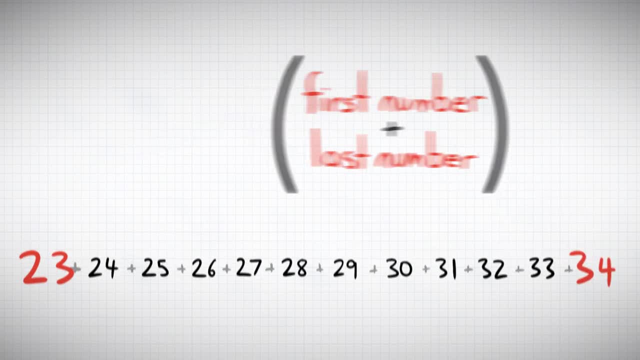 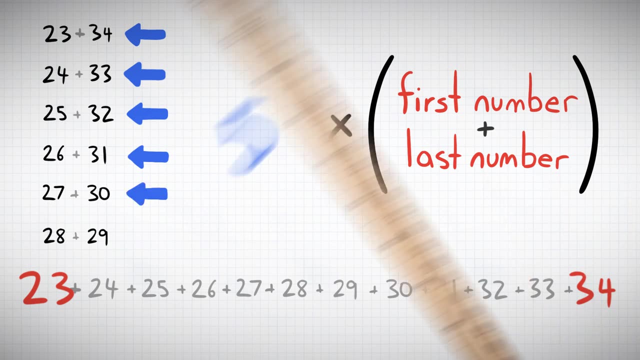 add the last number to get the value of the pairs. Then we just have to multiply that by the number of pairs. So you know 1,, 2,, 3,, 4.. Counting is for Philistines. And what if there's too many numbers to count? 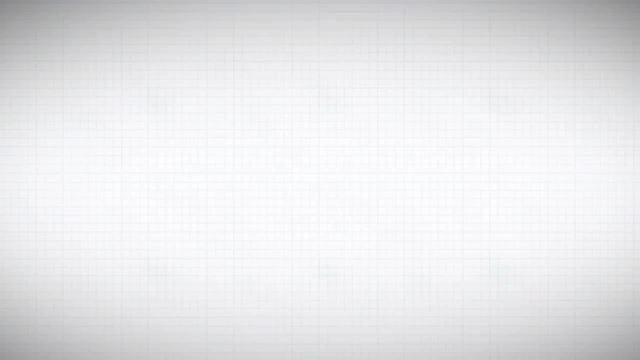 You can't count them. There's too many, So let's find a better way to do it. Let's say we wanted to count the number of numbers from 3 to 6. And we know the answer is 4.. So let's see if we can make 4 from the numbers we're working with: 3 and 6.. 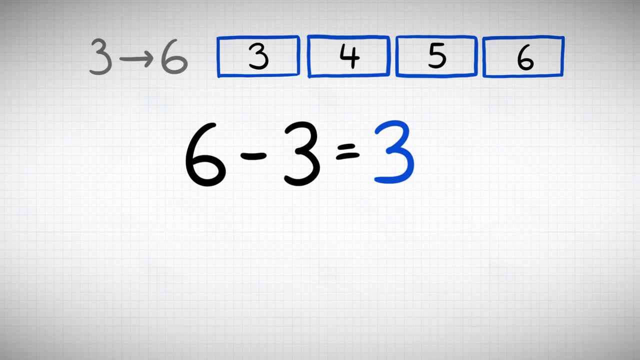 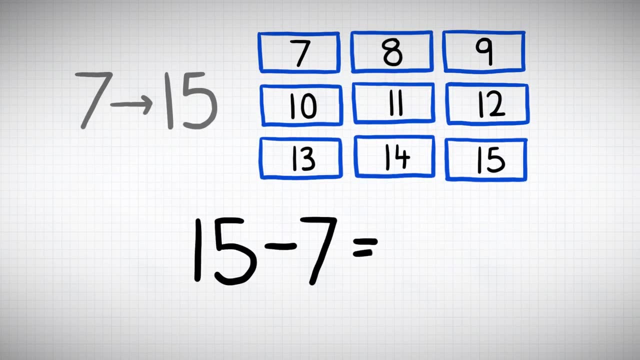 Could start with subtracting them, But when we subtract them we get 1 away. If we were counting the number of numbers from 7 to 15, there's 9 numbers, But if we subtract them, we also get 1 away. 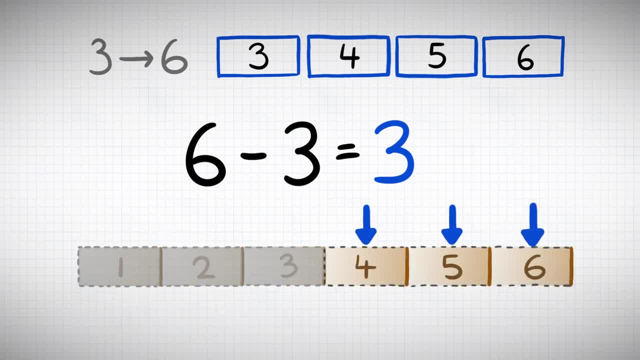 Because subtraction is giving us the difference between the two numbers, Whereas because of the specific way we've ordered the problem, we want to count from something to something. we want to take account of that first number that gets subtracted. So to make up for the number that gets lost, we just have to add 1.. 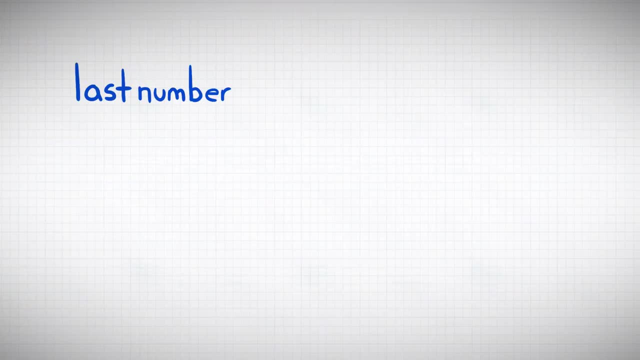 And that's it really Okay. So we take the last number, subtract the first number to get the difference between them. Add 1 to make up for that 1 that gets lost in the subtraction. Divide by 2 to go from having the number of numbers to having the number of pairs. 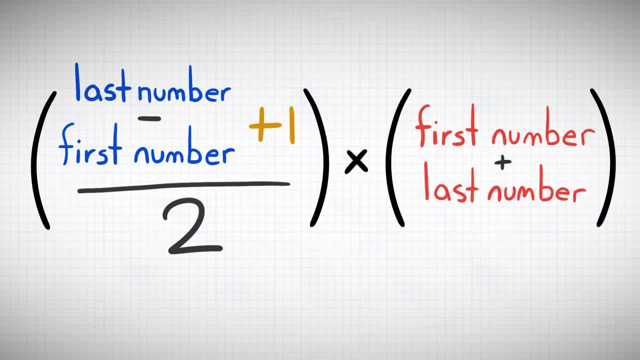 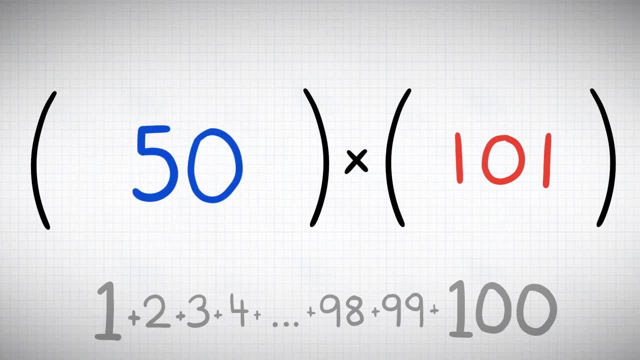 And then multiply that number of pairs by the value of the pairs. So if you want to add up all the numbers from 1 to 100, we go shabadoo Womp, whoosh, whoosh, waka the answer. 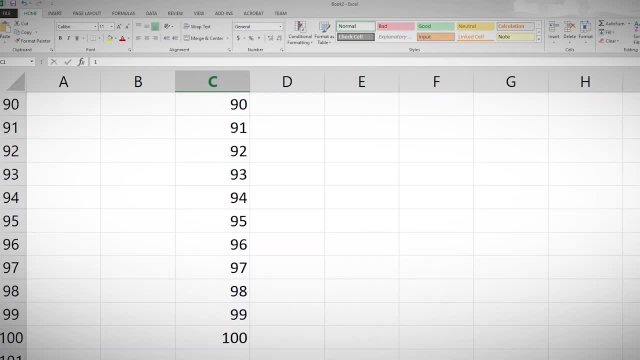 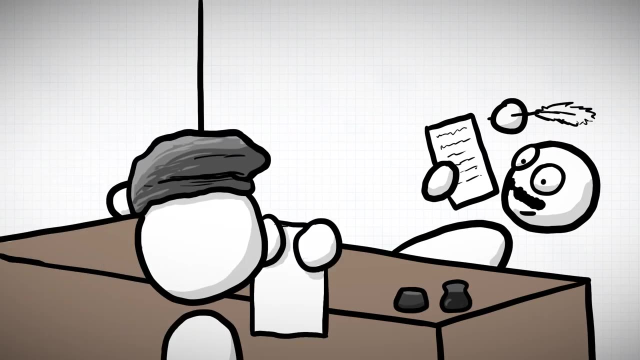 And we can check that with a computer. I guess computers are okay- I'm sorry for calling you basement dwellers- And so he came up with the answer really fast, and the teacher was like What. He just couldn't believe it. 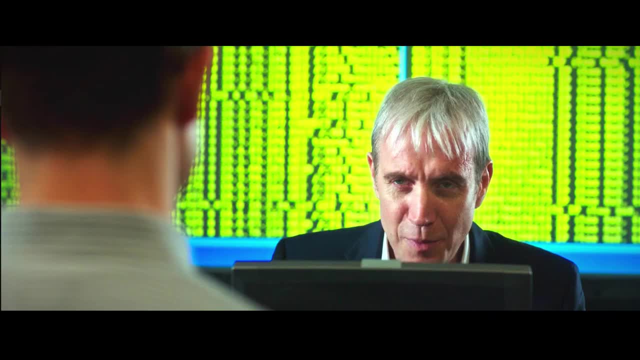 You know, kind of like that scene in a movie. I'm done What? Oh, You know, you don't have to tell me when you finished a portion of it, you brown-nosing little shi- No, I'm done the whole thing. 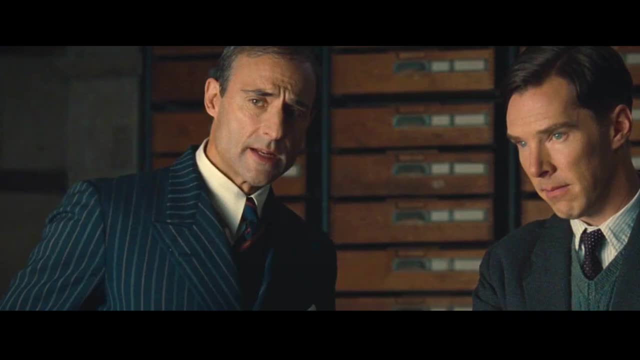 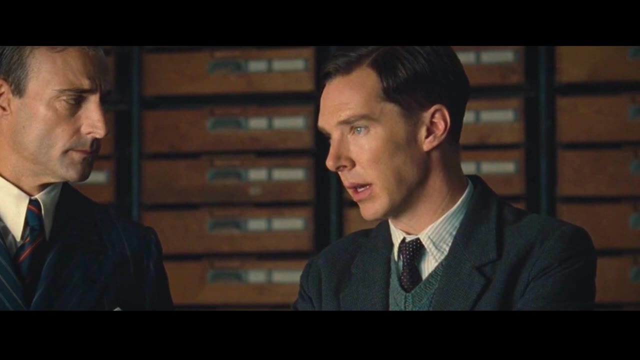 What Is this test even possible? Do they have enough time to get this done? I'm so mysterious. No, no, no, it's just a test in problem solving. I want to see how they approach the task, Because that's really the key in what we're looking for. 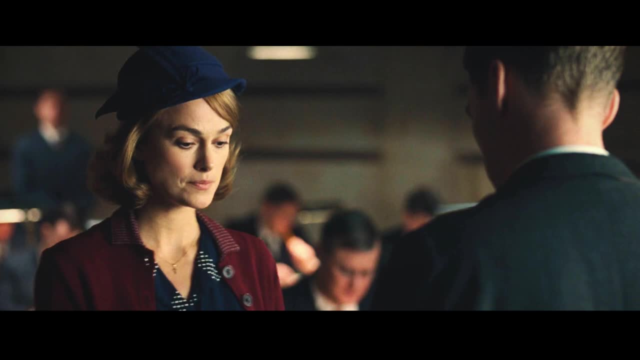 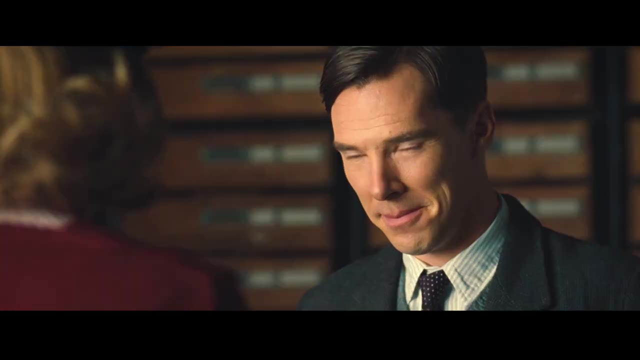 I am no man, What I mean, I'm done, What I guess. it just goes to show When, sometimes, sometimes when you don't expect anything of sometimes the people you don't expect, and that's the equation, And we can use it on really really long sequences if you wanted. 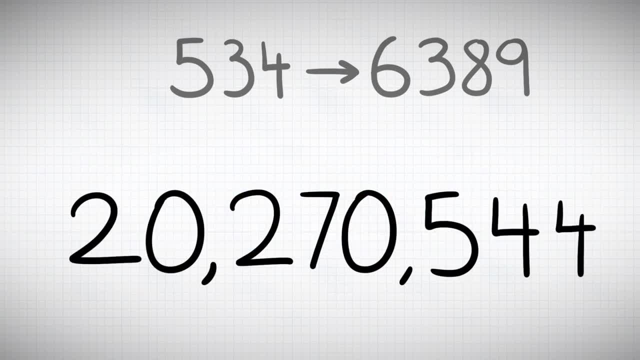 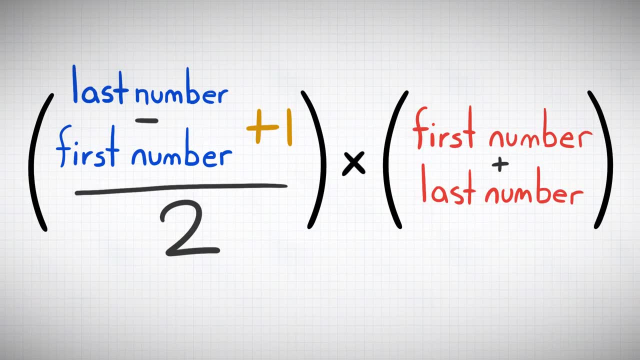 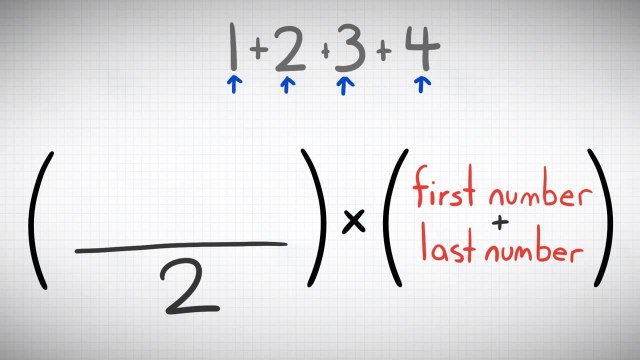 Shoop Whoosh, Shoop Whoosh, And we can check that The equation he came up with was actually easier, Because when you're counting from one to something you can kind of skip all this nonsense. There's four numbers when you're counting from one to four. 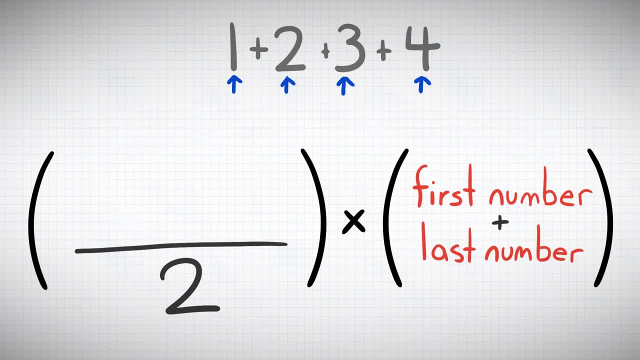 There's a hundred numbers when you're counting from one to a hundred, So we don't have to calculate the number of numbers. That last number is just the number of numbers. Also, the first number when you're counting from one to something is just going to be one.